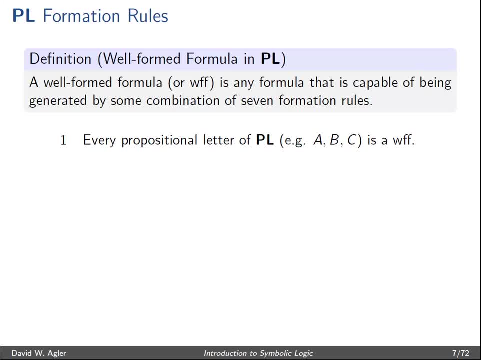 is a WOOF. So if you remember, the letters of propositional logic or the propositional letters are any uppercase Roman letter with or without numerical subscripts. So simply by writing an A or a B or a C or an F sub 5, we have formed a well-formed formula. Second, 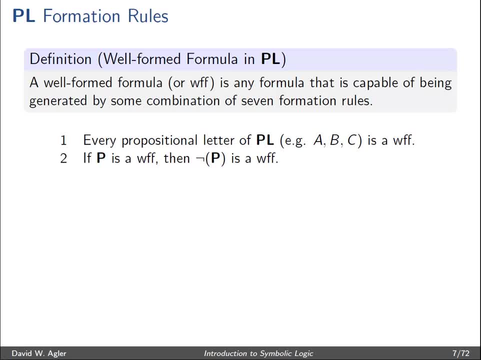 if we have a formula that meets the criteria of being a WOOF, then we can form another more complex formula by putting parentheses around it and the sign for negation to the left of it. Third, if we have two formulas that meet the criteria or standard of being woofs, then we can form a new, more complex formula by putting parentheses around both of the formulas and putting the caret or sign for and between them. 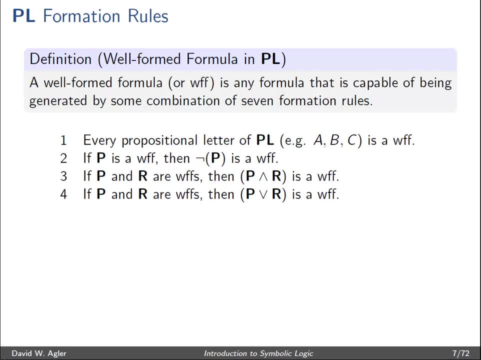 Similarly, if we have a P and an R or some combination of well-formed formulas, we can put the sign for V between it and the open and close parentheses around it, and we formed a woof. 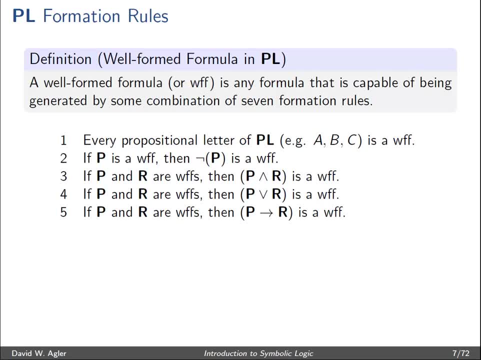 If we have P and R and those formulas are both woofs, then we can form another woof by putting the right arrow between it and parentheses around it, and the same thing is true for the double arrow. If P and R are woofs, then we can put the double arrow between them, parentheses around it, and the result is a woof. 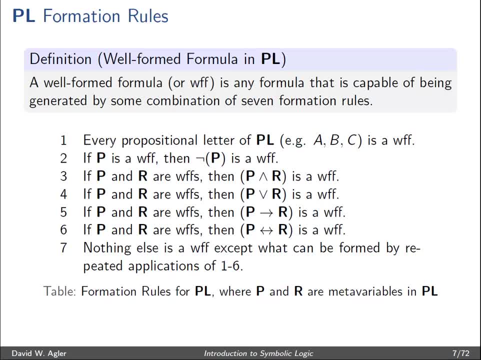 The final rule just indicates that rules one through six are all there are. There's no sneaky, hidden, additional rules that will form well-formed formulas, and all well-formed formulas in the language of propositional logic can be formed by these six rules. 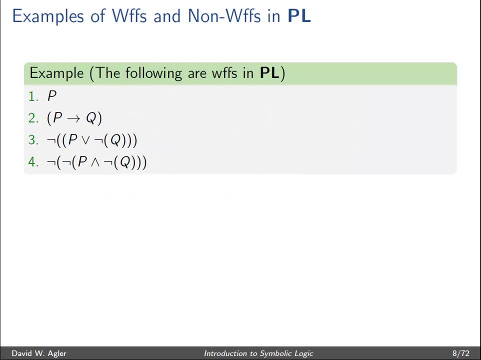 So let's look at a couple examples of woofs and not woofs in the language of propositional logic. 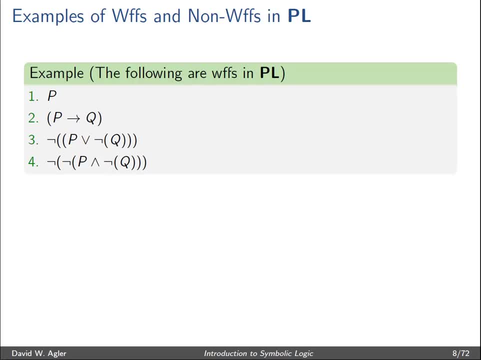 In the first case, we just have P, and this is a woof simply by the fact that every two formulas are woofs. Every propositional letter is a woof. 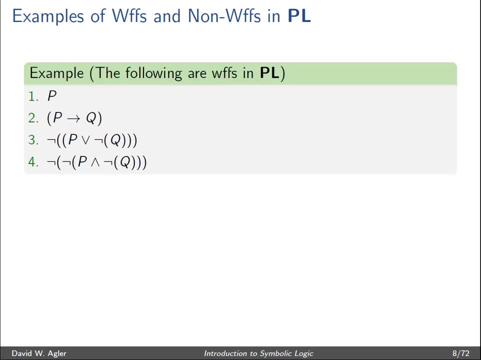 Second, we have a formula that looks a little bit more complex on number two. We know that both P and Q in their own right are woofs because every propositional letter is a woof, and one of the rules allows us to form this open parentheses P right arrow Q close parentheses because since P is a woof and Q is a woof, we can put the right arrow between them and parentheses, and we can put the right arrow between them and parentheses around them. 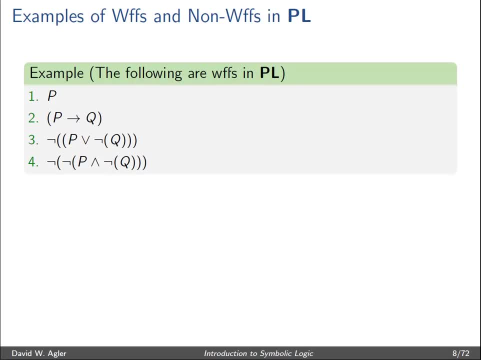 Now, three and four are a more complex example. 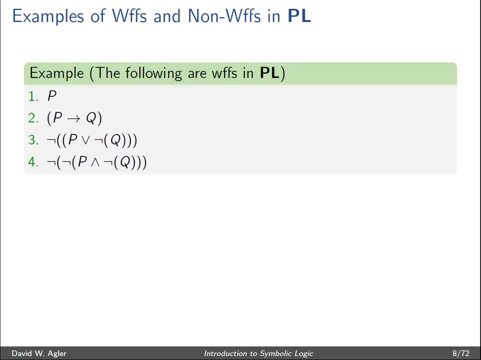 In the case of three, you'll notice that P on its own is a woof, Q on its own is a woof, but what we have here is a formula with a couple different operators. So let's start from the basics and work our way up. We know that Q is a woof. We also know that we can form a more complex woof by putting parentheses around Q, and then negation to the left of Q. So, we also know that not Q is a woof. Well, if we know that P is a woof, and we know that not Q is a woof, we also have a rule that allows us to take two well-formed formulas and put them together and put the sign for V or the OR sign between them and put parentheses around it. 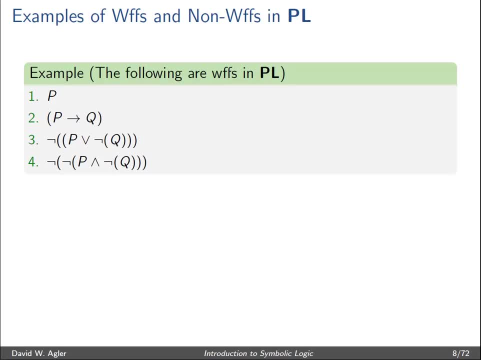 And that's what we have as part of the formula line three. 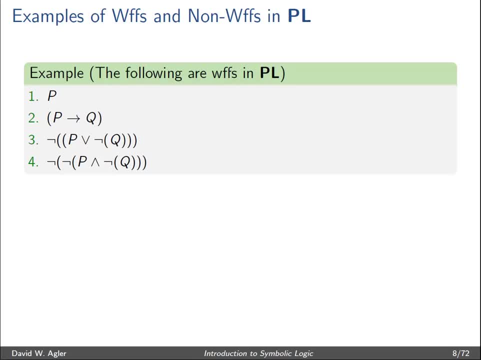 Now, the last part, sort of states that, well, if we know that open parentheses P or not Q is a woof, 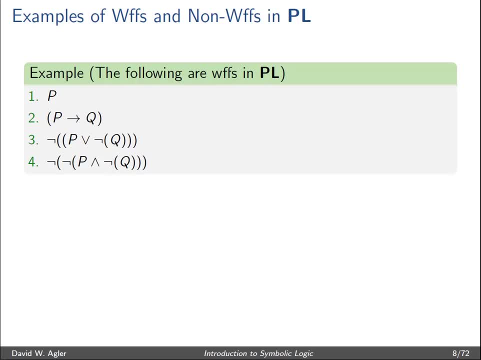 then we can put parentheses around that whole well-formed formula and then put a negation to the left and their result will be a woof. 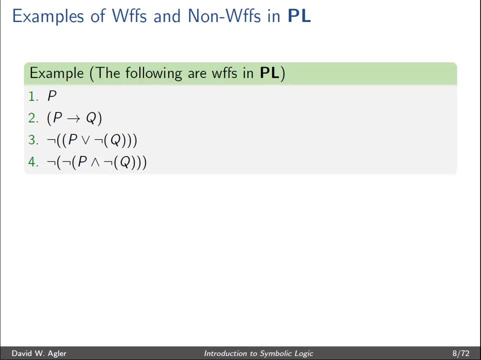 So, the general point is that we can use the formation rules in a step-by-step manner to create increasingly complex woofs. 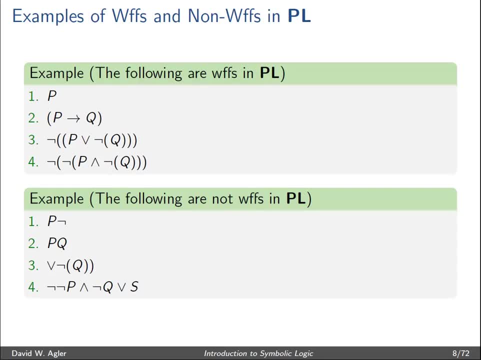 So, here are a couple examples of formulas that are definitely not woofs. In the first example, 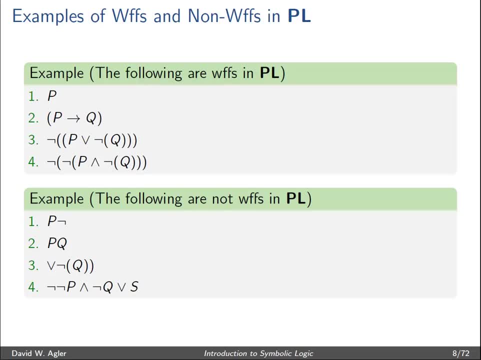 you notice that the negation or the sign for not is off to the right, and so this would not be an acceptable use of the rule that allows us to form not some well-formed formula 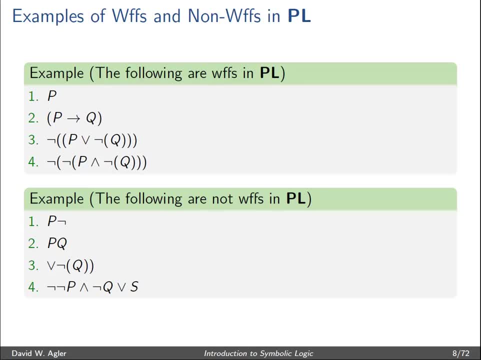 because that application of the rule states that you put parentheses around the well-formed formula and put the negation to the left, not to the right. 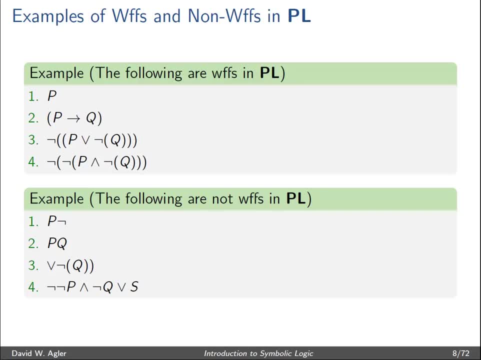 In the second example, you notice that there are just two propositional letters side by side. Now, there's no formation rule that allows us to do this, and so that combination of characters is not a woof. 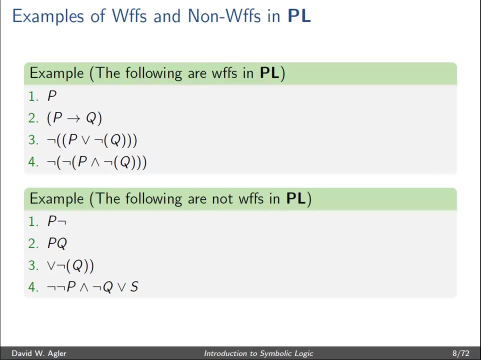 And the same holds true for examples three and four. These are not woofs because there's no combination of the formation rules that would allow us to form these formulas. 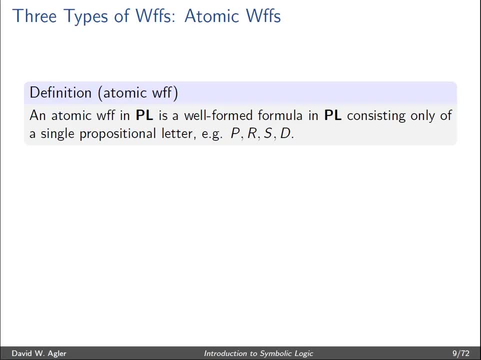 Now, lastly, I want to talk about three different types of well-formed formulas. The first is an atomic woof. 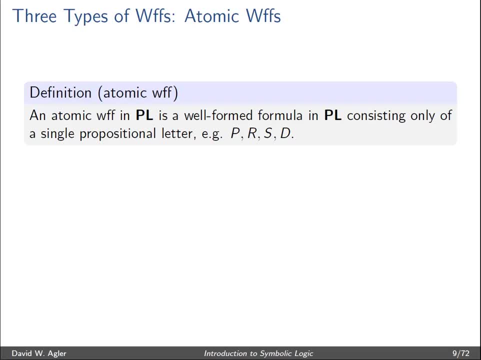 An atomic woof is any well-formed formula consisting only of a single propositional letter. And so, here are a couple examples of those. Let's look at some examples of atomic woofs in the language of propositional logic. P, Q, A, they're all single propositional letters, and so they meet the standard of being an atomic woof. 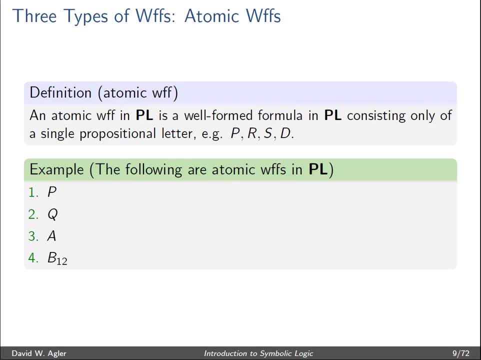 Similarly, B sub 12 is a propositional letter, and so it meets the standard of being an atomic woof. 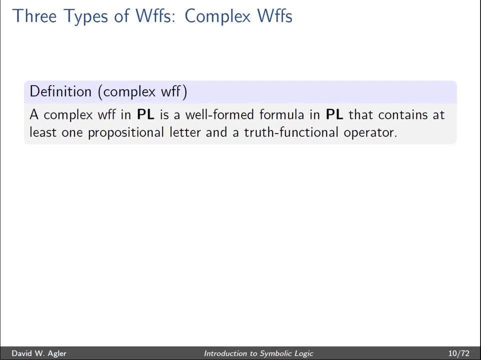 The second type of woof I want to talk about are complex woofs. Now, a complex woof is essentially any well-formed formula that has at least one truth-functional operator. Now, if you don't know what a truth-functional operator is, 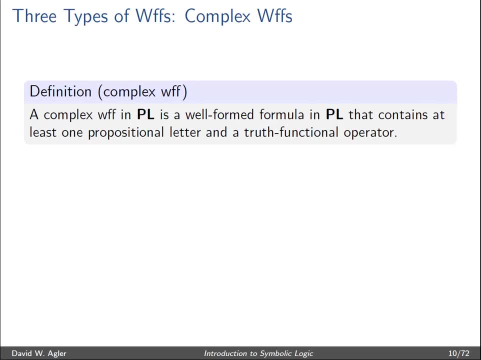 then I suggest you take a look at an earlier video that I'll put in the description below that indicates the symbols and characters of the language of propositional logic. So, let's take a look at a couple examples. 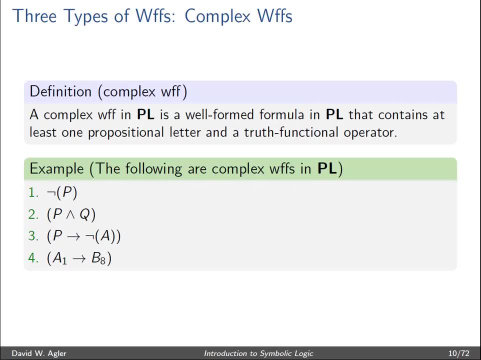 In the first example, you see not P has at least one truth-functional operator, and it's also a well-formed formula. So, since it meets both of these standards or criteria, then it's a woof. 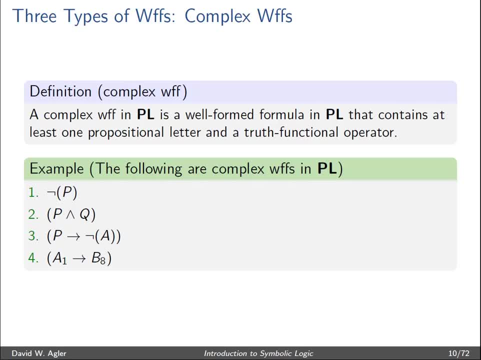 The same thing with line two, three, and four. Each one of these has at least one well-formed formula, and all three of these, or actually all four of the examples, are a well-formed formula. 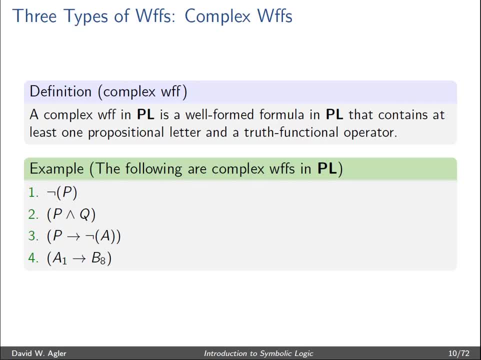 So, it meets all the criteria necessary to be a complex woof. 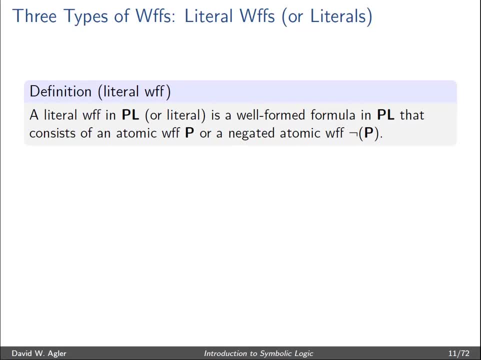 The last type of woof I want to talk about is known as a literal woof, or more simply, a literal. Now, this is any woof that is either an atomic woof or a negated atomic woof. So, let's look at some examples. So, in the case of P, all by itself, this is an atomic woof because every propositional letter is an atomic woof. Now, since it's an atomic woof, it's also a literal woof, since a literal woof is either an atomic woof or a negated atomic woof. 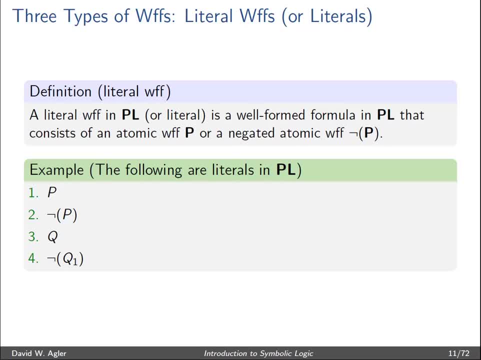 In the case of two, and then also four, you notice that there is the negation of a propositional letter. That is, there's the negation or not of an atomic woof, and so both of these, number two and four, as well as three, are all literal woofs. 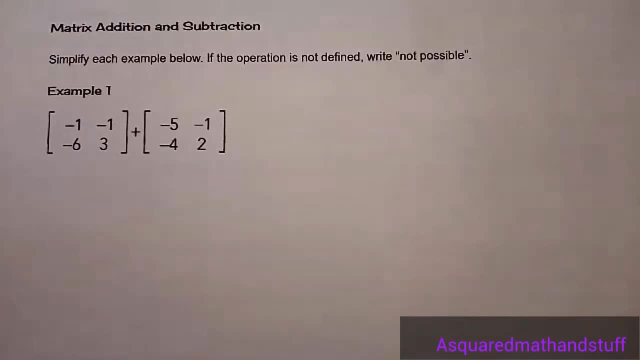 Hello math friends and welcome back to A Squared Math and Stuff. Today's examples are going to focus on matrix addition and subtraction. One thing about matrix addition and subtraction is you can only add or subtract matrices that have the same dimensions. In this first example, 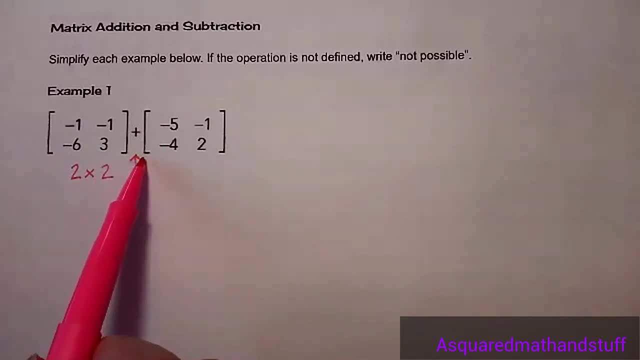 here we have a 2 by 2 matrix and we are adding that to another 2 by 2 matrix. So this is possible, and when we add these together we add corresponding positions together. In other words, we're going to take this negative 1 and add it to the negative 5, and then we'll take row 1. 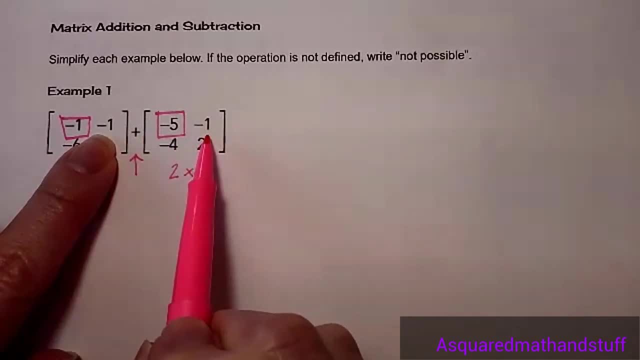 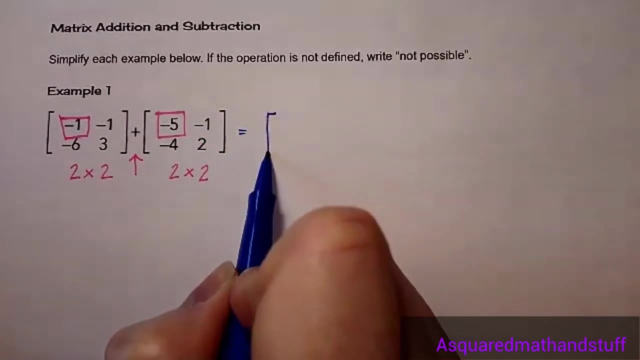 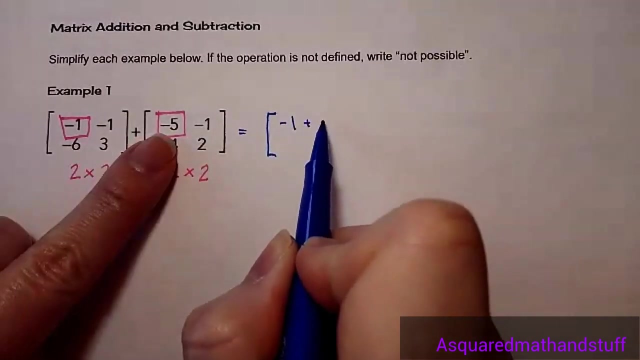 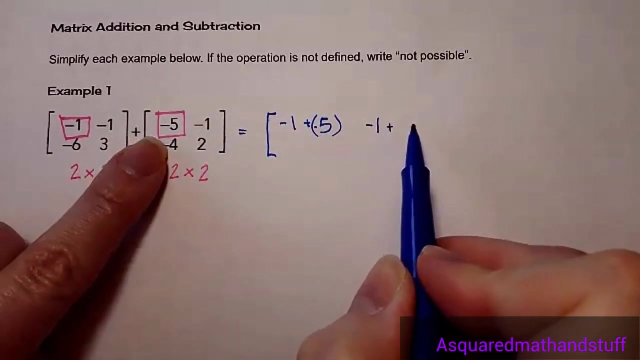 column 2 of this first matrix. add it to row 1, column 2 of the second matrix. So let's go ahead and write this out, Combining what we are adding and writing it into one matrix. we have our negative 1 plus the negative 5, and then we have a negative 1 plus another negative 1.. Going down to row 2, we 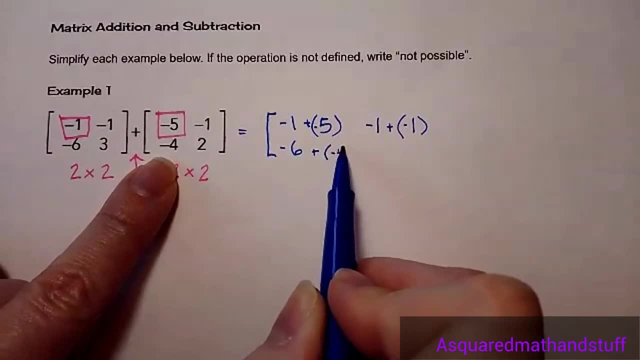 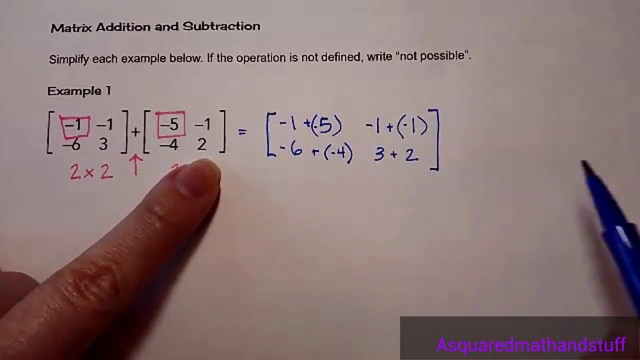 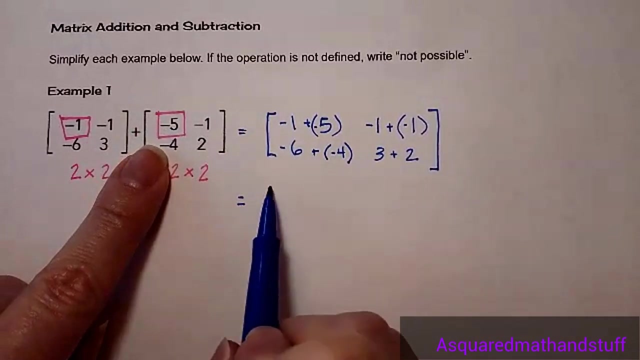 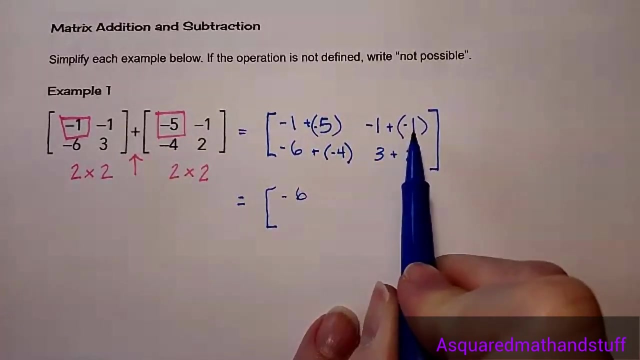 have a negative 6 plus negative 4 and then finally we have 3 plus 2.. Add these values together and we will get our final matrix after adding these two original that we were given. Negative 1 plus a negative 5 gives us negative 6.. Negative 1 plus a negative 1 gives us negative 2.. 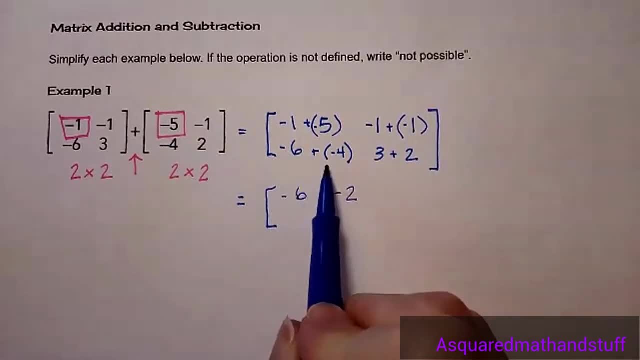 Negative 6 plus negative 4, negative 10, and then lastly, here we have a 3 plus a 2 gives us positive 5.. So that is the final answer for this first example here, when we add 2 by 2's together, The next example.